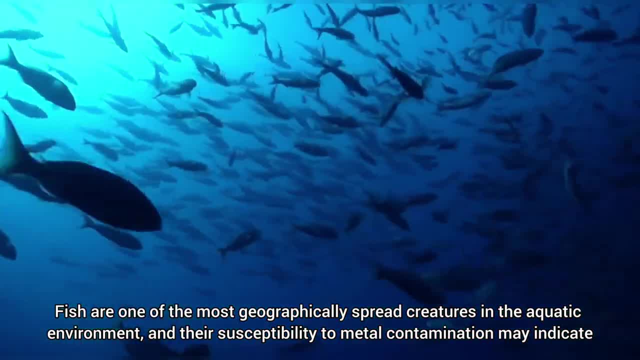 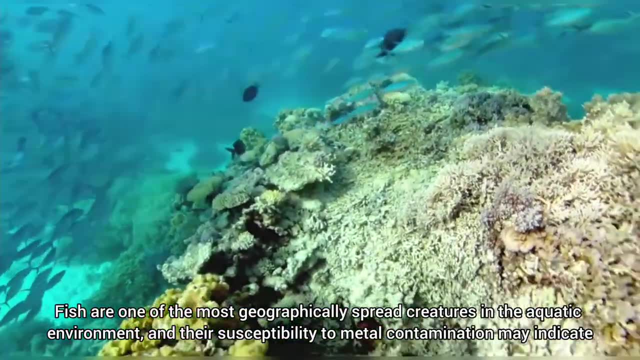 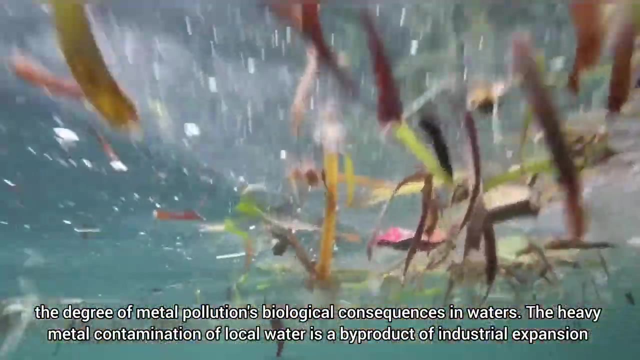 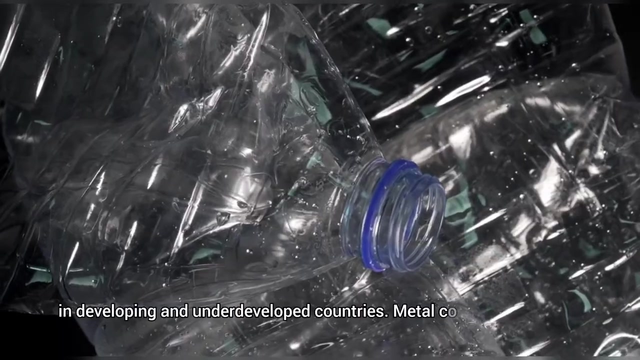 Fish are one of the most geographically separate creatures in the aquatic environment and their susceptibility to metal contamination may increase. Heavy metal contamination may indicate the degree of metal pollutants' biological consequences in water. The heavy metal contamination of local water is a by-product of industrial expansion in the developing and underdeveloped countries. 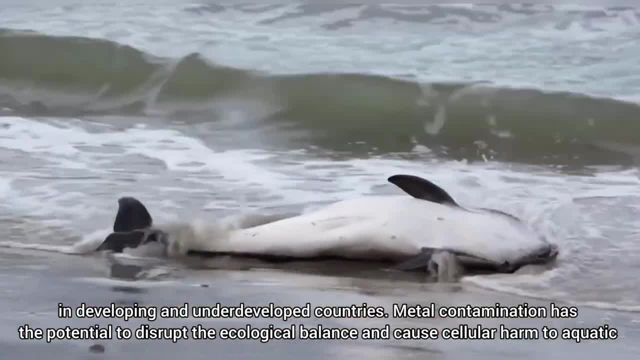 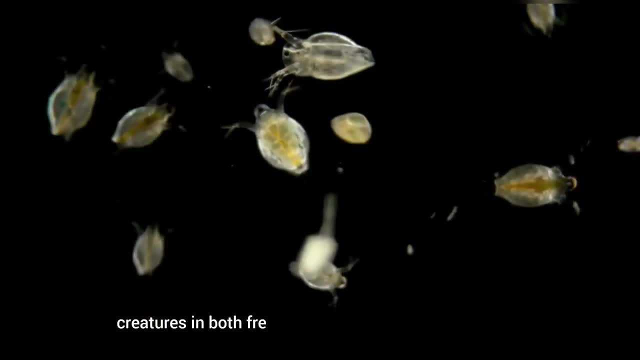 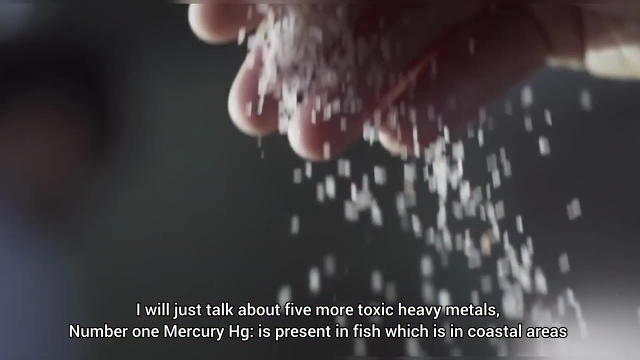 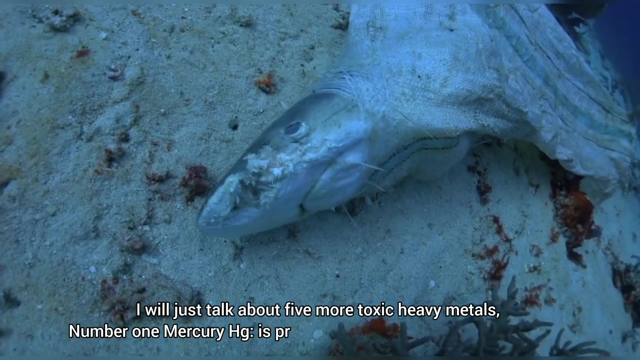 Metal contamination has the potential to disrupt the ecological balance and cause cellular harm to aquatic creatures in both fresh and marine environments. I will just tell you a few things. I will tell about five more toxic heavy metals. Number one: mercury. Mercury is present in fish which is in coastal areas within two to three miles from coast. 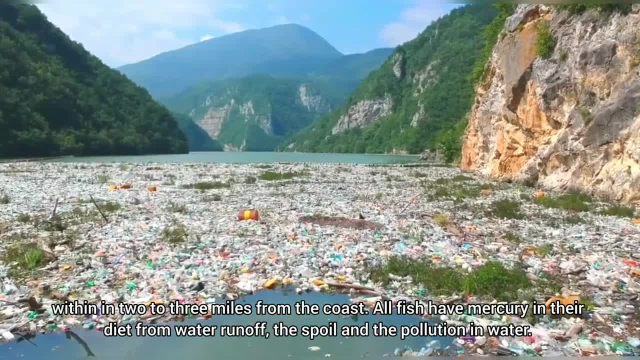 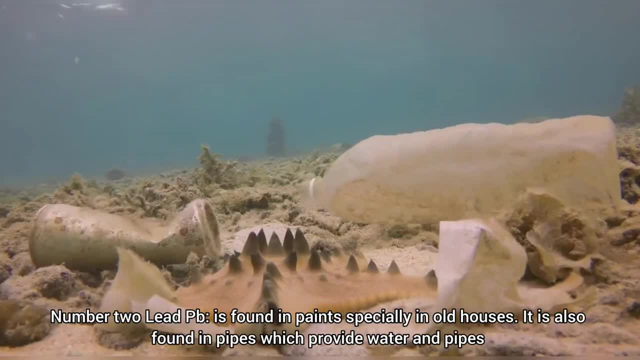 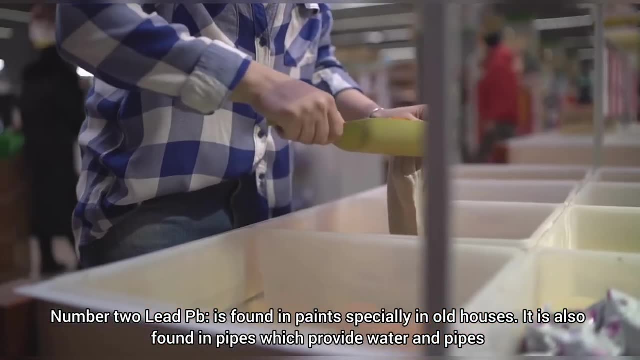 All fishes have mercury in their diet. from water runoff, this oil and pollution in water Number second, lead. Lead is found in paints, especially in old houses. It is also found in pipes which provide water and pipes which are used for the wastewater, and in twice. 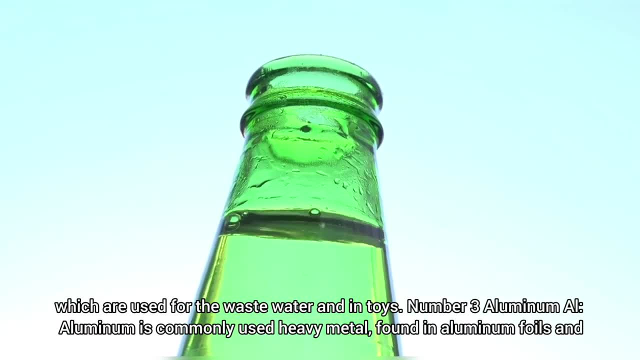 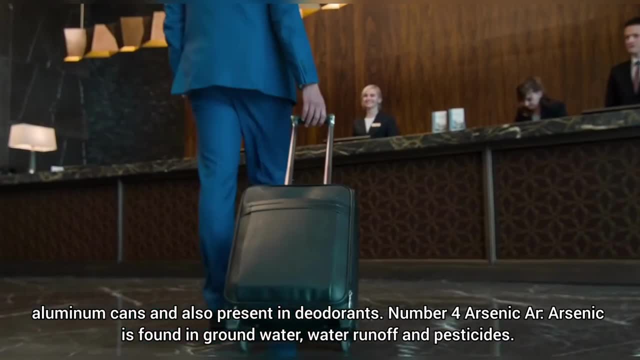 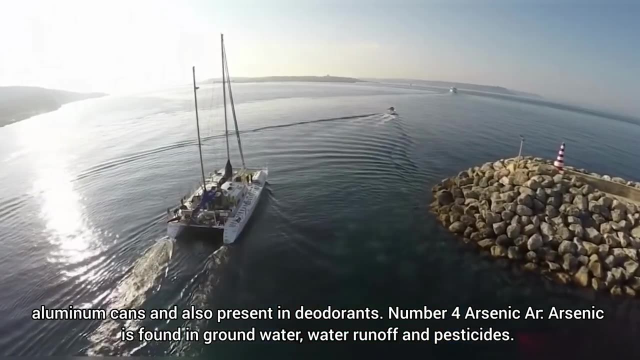 Number third is aluminum. Aluminum, commonly used is heavy metal found in aluminum foil, aluminum cans and also present in deodorants. Number four is arsenic. Arsenic is found in groundwater, water, runoff and pesticides. Number five: cadmium. 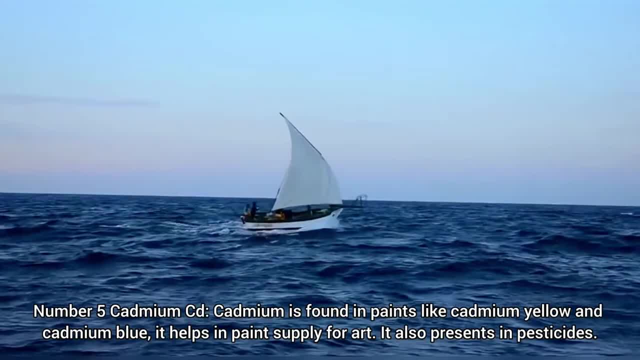 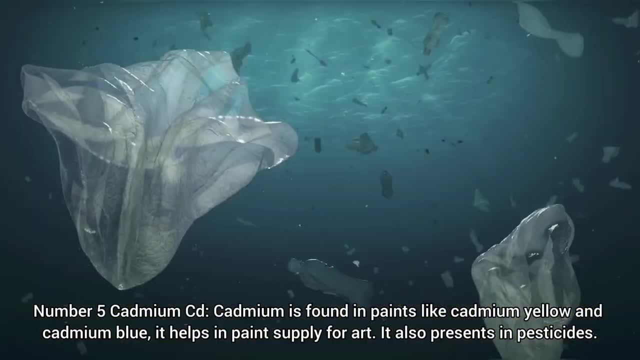 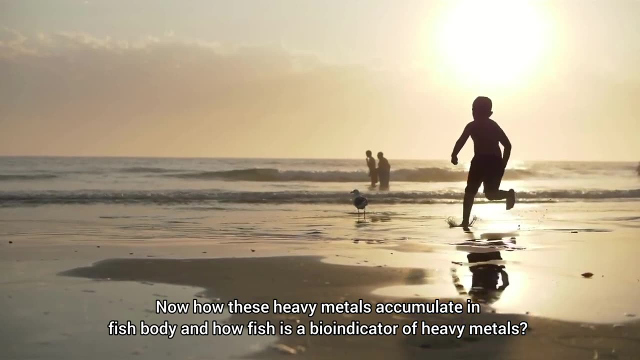 Cadmium is found in paints like cadmium yellow and cadmium blue. It helps in paint supply for art. It is also found in pesticides. Now how these heavy metals accumulate in fish body and how fish is a bio-indicator of heavy metals. 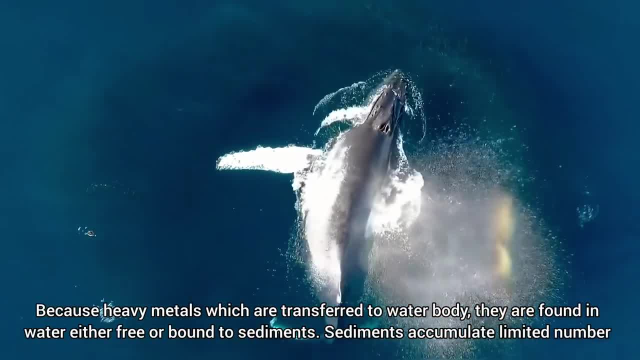 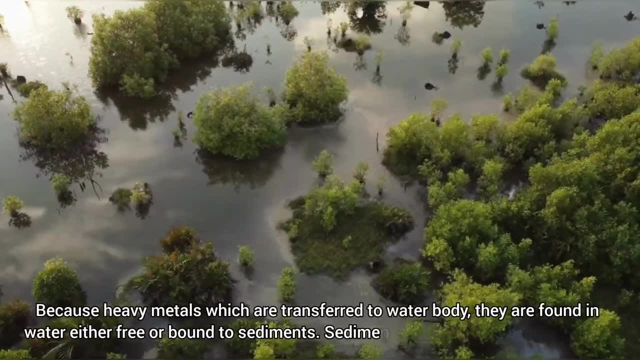 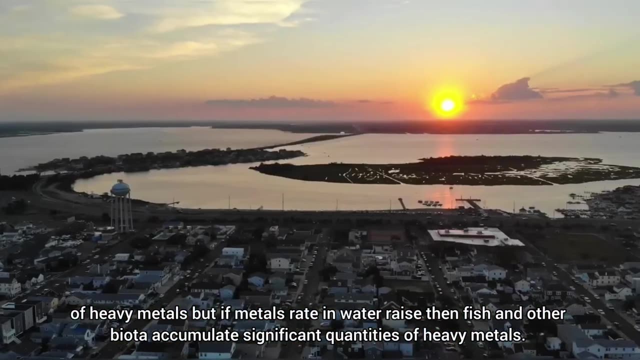 Because heavy metals which are transferred to water body. they are found either free or bound to sediments. Sediments accumulate limited amount, but if heavy metal rates in water raise, then fish or other biota accumulate significant quantities of heavy metals. Fish uptake heavy metals.